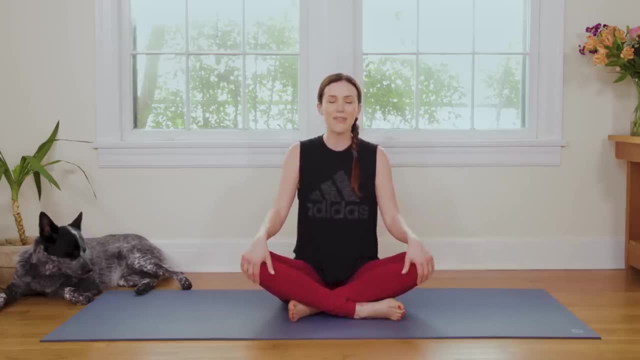 We're gonna sit up nice and tall Right away, take a deep breath in And, as you exhale, just relax your shoulders down, away from the ears arriving here for your ten minute awesome practice. Inhale in again through the nose. 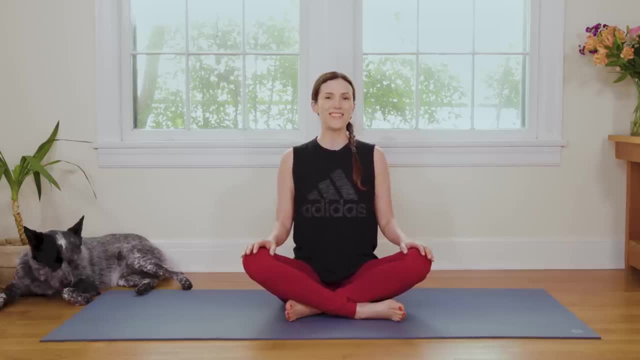 Exhale, relax the shoulders down And, for this next cycle of breath, go ahead and close your eyes. Here we go: big breath in And long breath out, relaxing the shoulders down, Allowing yourself to arrive here in the moment. 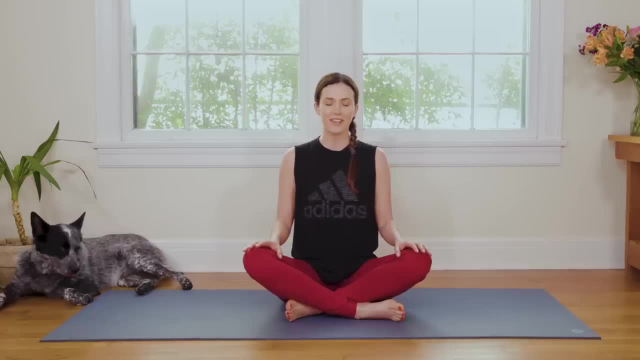 I always say a little goes a long way And that it shall Go ahead and open your eyes. We're gonna bring the fingertips to kiss the tops of the shoulders, moving with the breath. Inhale, send the elbows forward, Let the elbows kiss together or reach towards each other. 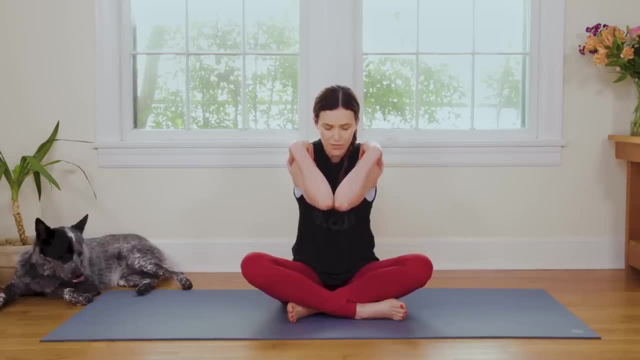 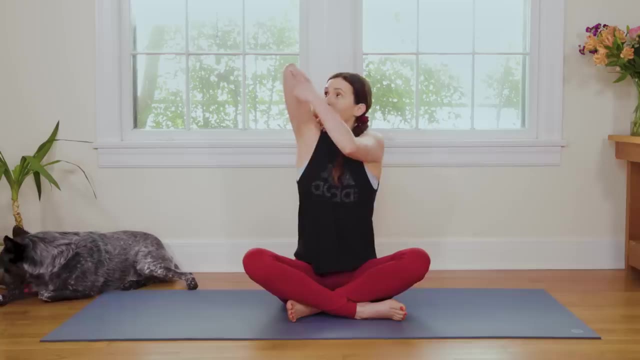 Feel that stretch in the upper back body And draw your navel in, Then slowly continue the journey, taking the elbows all the way up: Reach, reach, reach. Think of this long, beautiful stretch from elbow to shoulder and shoulder to waistline. 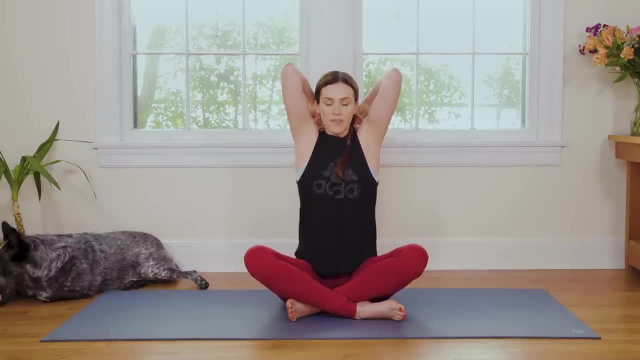 So we're really lifting up out of the waist. Great, then continue the journey. Carve a line with your elbows all the way back, Opening up through the pecs, the chest. Imagine you're pinching a pencil between your shoulder blades. 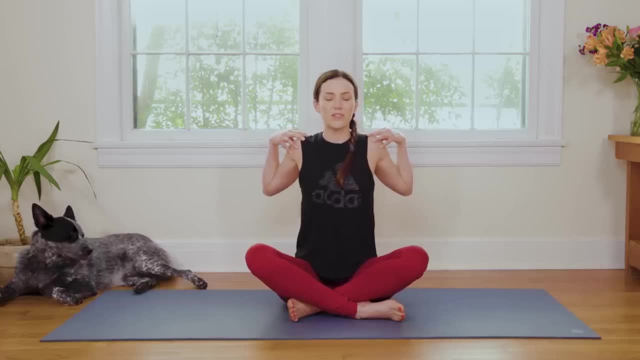 here, really retracting back Elbows, reaching towards the center of the back body And then all the way down. Tag a lot of weight in your elbows, Feel this beautiful stretch, Inhale, Stretch through the neck. You can even gently nod the head. yes, here. 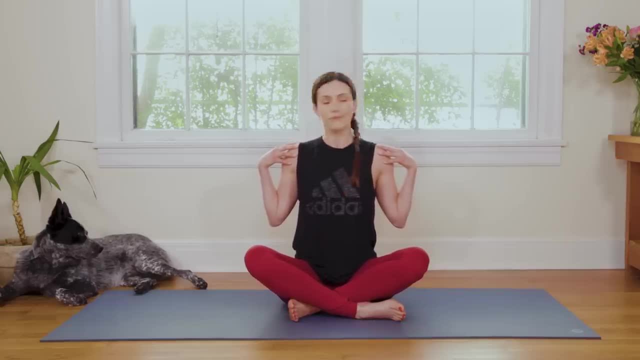 And then no Great, then we're just gonna do the same thing, but with a little more fluidity. Here we go: elbows kiss together, Deep breath, reach it all the way up, Lift up out of the waistline Big stretch, take it around and back. 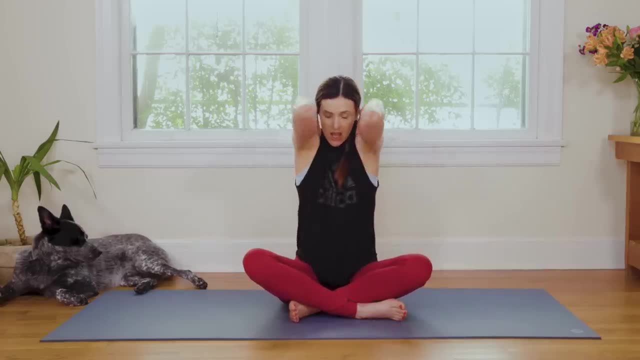 Again. inhale to reach forward, Feel the upper back, body stretch, Then lift up all the way up from the pelvic floor Around and back, And then one more. here we go, Big breath as you reach the elbows forward And up around and back. 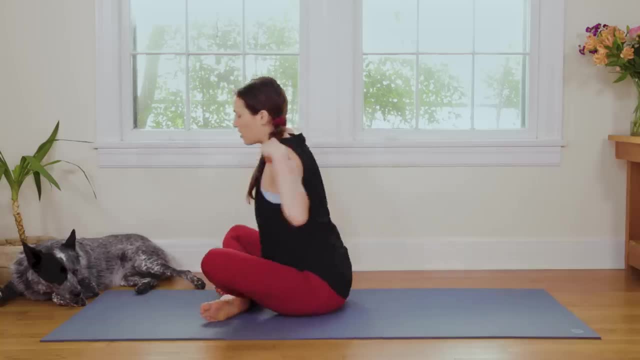 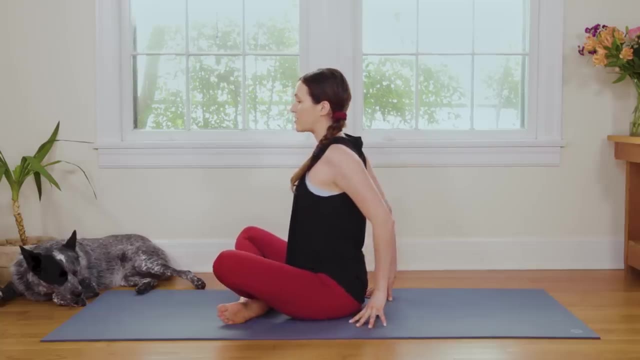 Now, this time when you're back, keep the heart lifted, Shoulder blades drawing together. You're gonna release the fingertips down. Fingers stay facing in towards your body and you're gonna bring the fingertips to kiss the earth, Squeeze the elbows back. 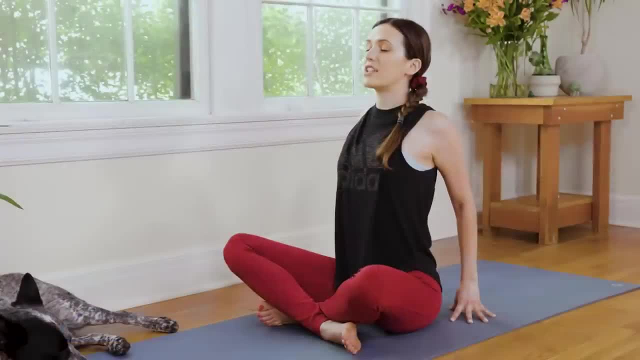 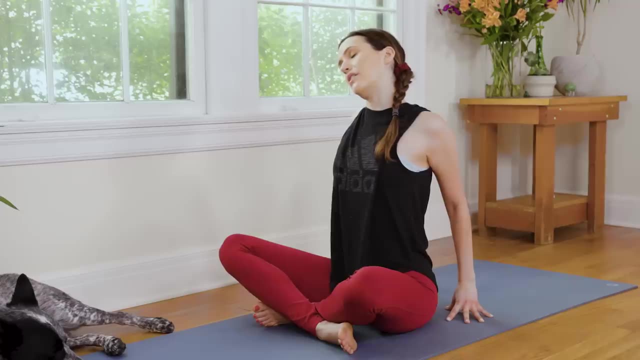 Inhale, lift the chest, Lift your sternum And then a gentle lift of the chin. Good, Beautiful Inhale in here. Exhale right ear over right shoulder, Breathe, Pressing into the fingertips. 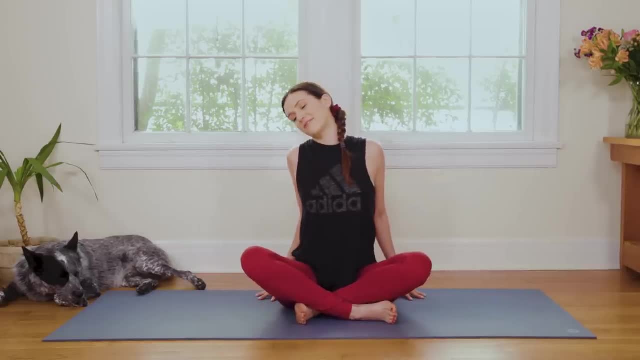 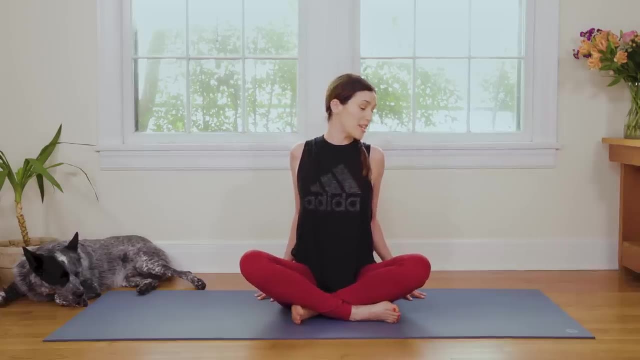 Drawing the shoulder blades together And then bring the head back to center And the left ear over left shoulder, Squeezing, actively, squeezing shoulder blades together. Upper back body engaged, Gorgeous, Bring it up, Release the hands, Palms come together. 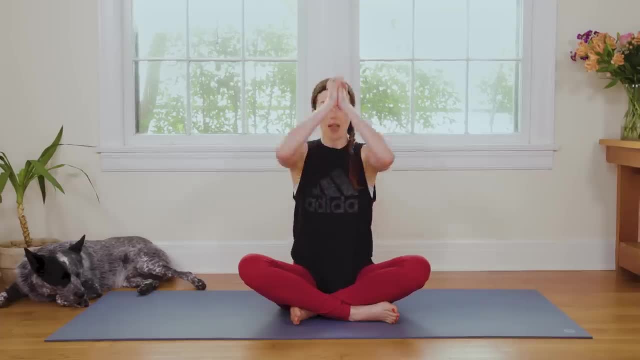 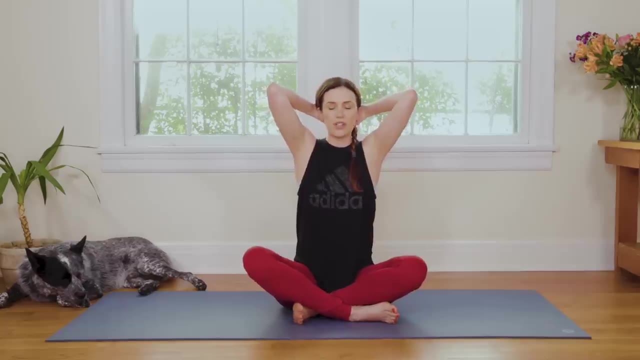 Namaste And release the fingers, You're gonna bring them all the way up and behind the head. Thumbs can extend to cradle the neck. You can even give yourself a little neck massage here, And then we're gonna inhale. 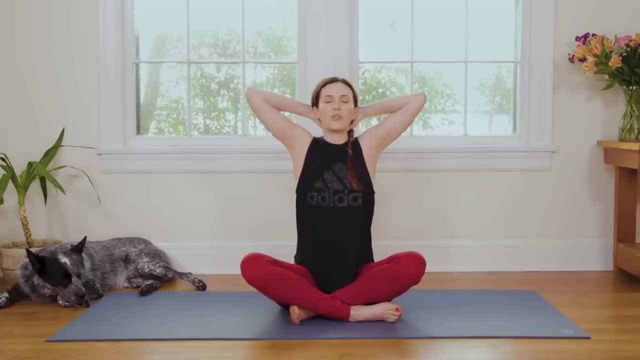 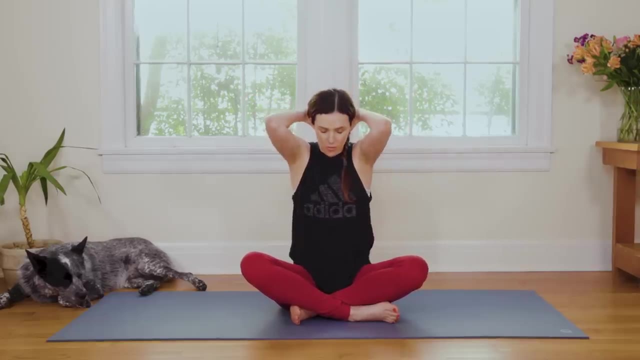 Lift up through the front body, Think Cobra. Exhale, draw the shoulder blades together again. Elbows nice and wide. Inhale in here. Exhale chin to chest. Elbows kiss together And you're not gonna actively press the hands against the head. 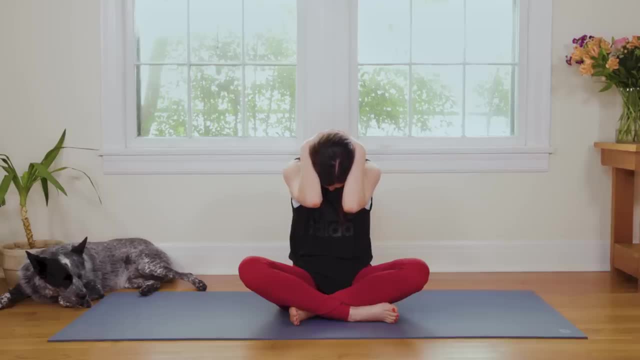 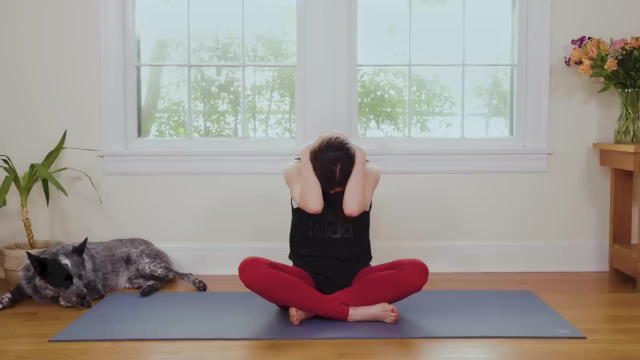 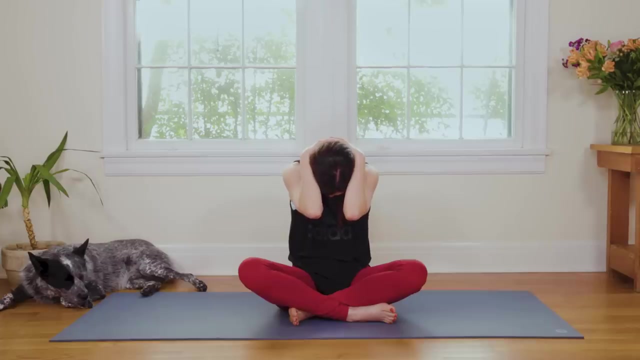 but just allow gravity, Ready to do the work here. Breathing So important that you bring the element of the breath into play. Take one more cycle of the breath here, In And out, And think of this as a blossoming. 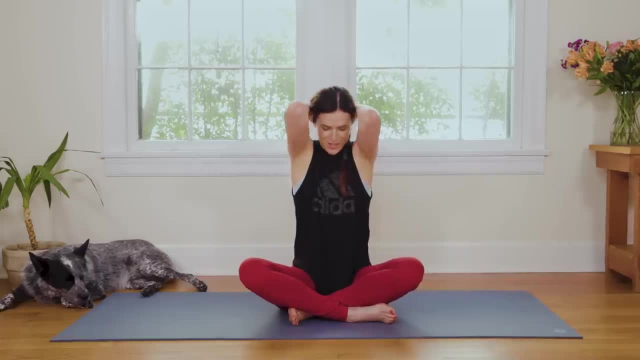 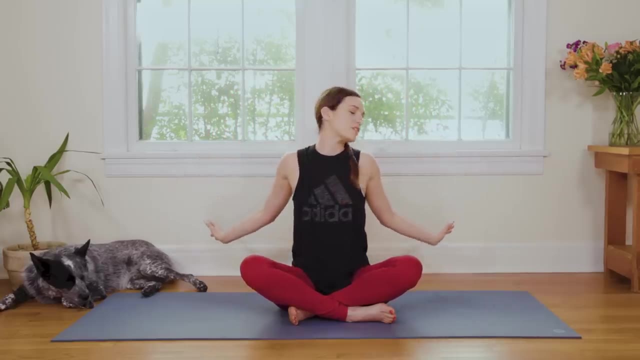 You're gonna slowly lift the chest, So take your time. basically Lift your heart, Open and then just release the fingertips: Big stretch any which way that feels good. Opening through the chest, Finding soft, easy movement through the neck- Awesome work. 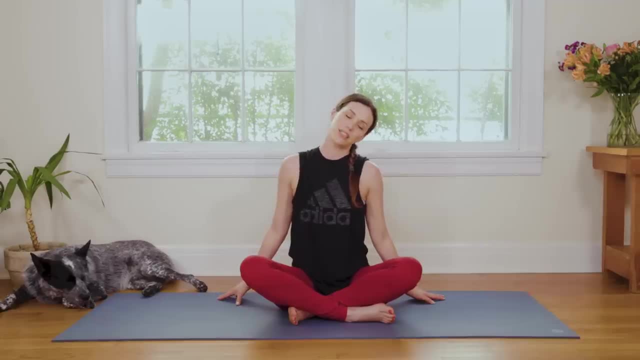 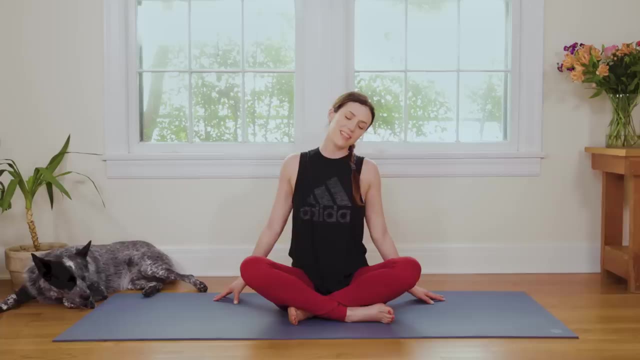 Okay, from here left ear to left shoulder. once again, Right fingertips are out. We're gonna inhale in. Exhale, draw the shoulder blades together, Inhale in again. You're gonna begin to lift up your right fingertips and flex. 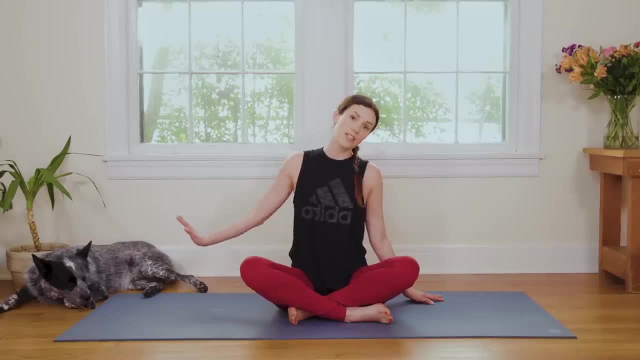 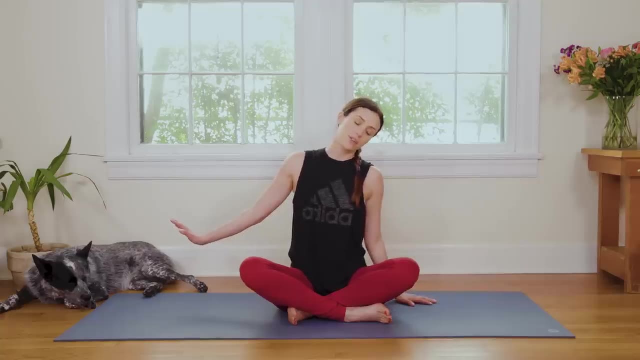 Right fingertips towards the sky, So we're pressing right hand into an imaginary wall. You're feeling a beautiful stretch between the right ear and right shoulder and the neck, The trapezius, The upper back body, still engaged as the heart lifts. 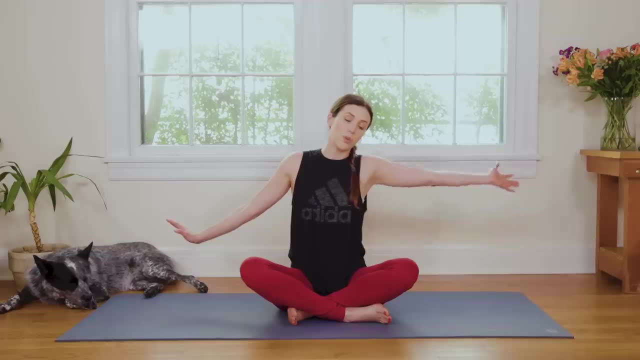 If you need a little more here, take your left fingertips, Gently, sweep them all the way up and over and right on the right ear here Just gently resting again, Not pressing, Letting gravity do the work. Notice if you're collapsing forward here. 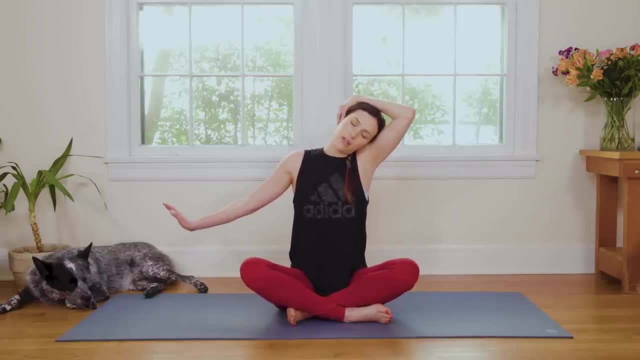 actively draw the shoulder blades together, Breathing deep here, and if it's too much you can just bring the fingertips down and if you need more, reach the fingertips all the way up. Big sensation, Great inhale in here. Exhale to gently unravel. 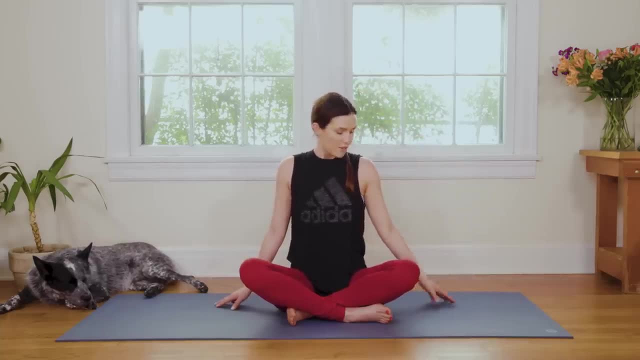 Release everything. Fingertips come to the earth. Great. whenever you're ready, right ear over, right shoulder, Breathing, Draw the shoulder blades together, Lift your heart. When you're ready, left fingertips, begin to levitate And then we'll flex. 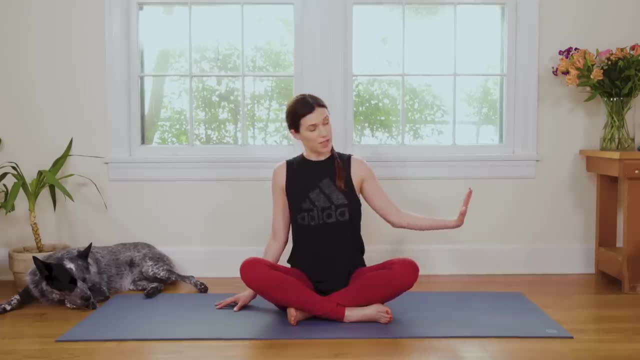 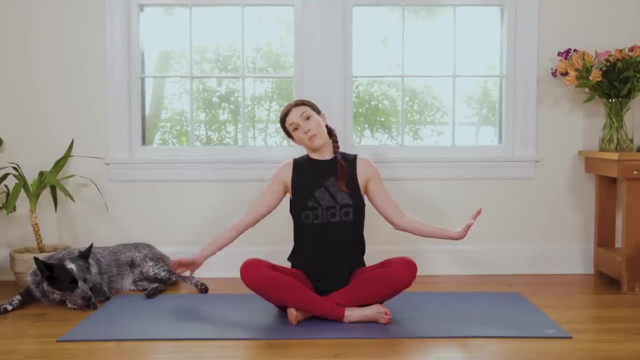 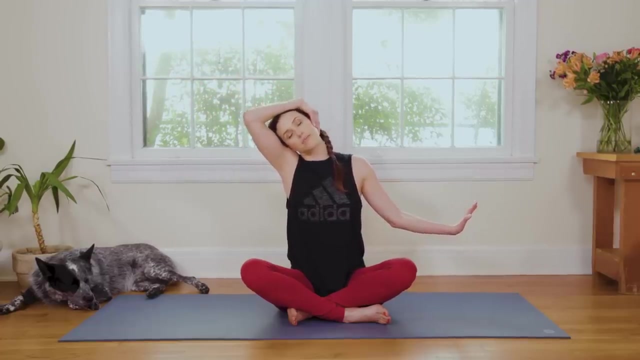 Pressing left palm away, Really reaching left fingertips towards your face. Keep the chin slightly lifted here, Interested in a little more. then you can take your right fingertips, sweep them all the way up and over and around to land gently on the left ear. 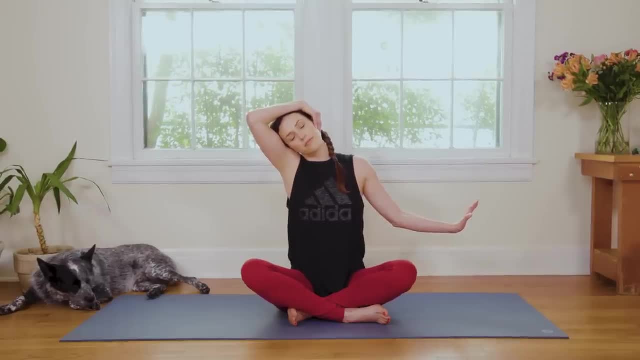 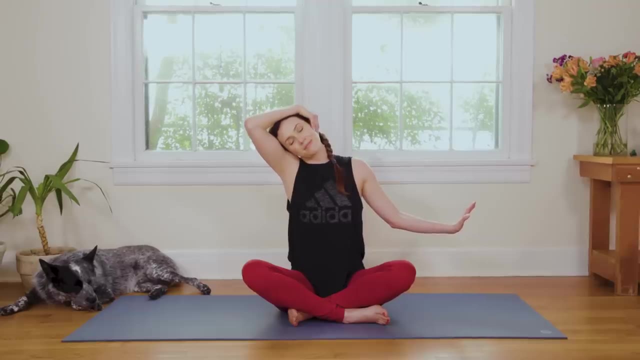 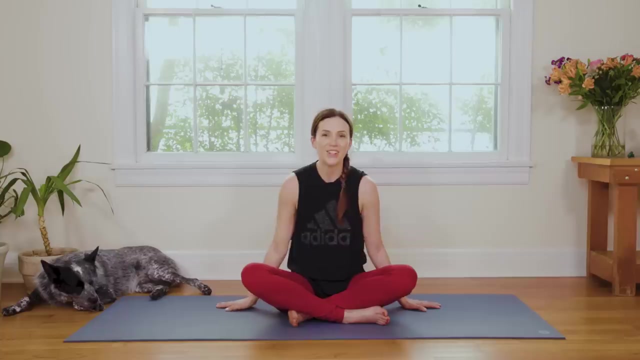 Breathe deep here. Take one more deep breath in and out- Awesome. Take one more cycle of breath in and out. Slowly begin to unravel both fingertips. Kiss the mat here On your next breath in, lift the shoulders up to the ears and then. 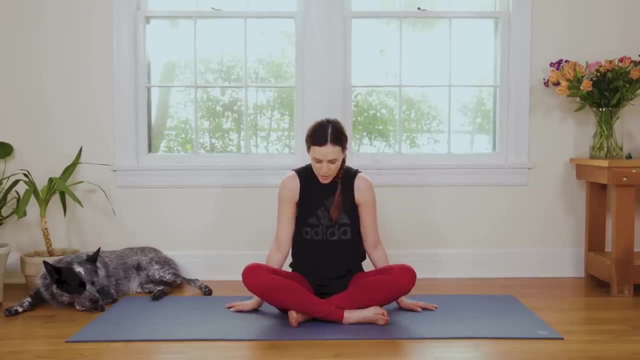 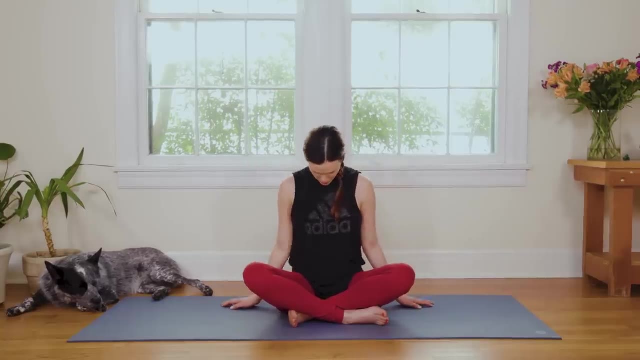 exhale, take them around and back and down. Twice more like that Inhale. reach them up, lift them up. Big breath in Exhale, around and down And once more big inhale Inhale. 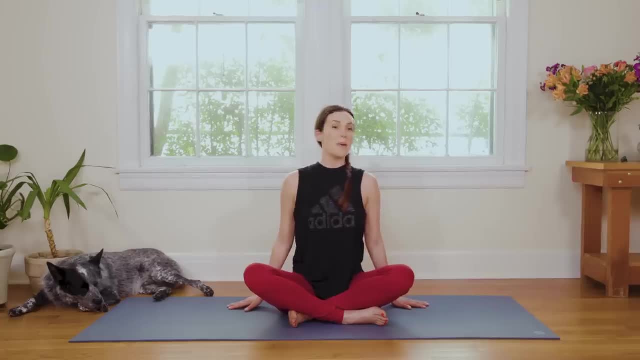 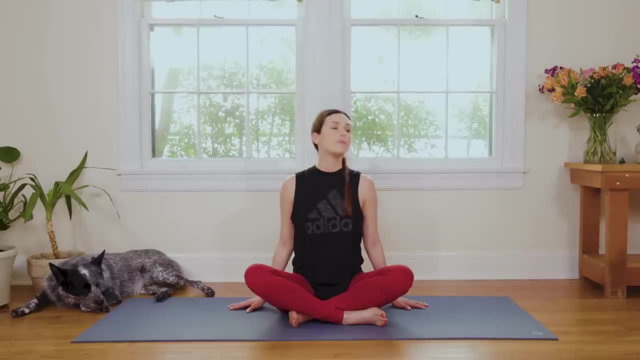 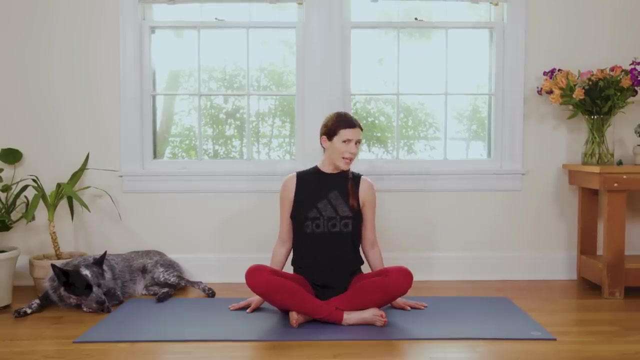 And exhale Awesome Baby little saucer-sized circles with the nose. You're gonna draw little baby circles one way And then let it grow a little bit bigger so we move from like a saucer to like a salad plate, if you will. 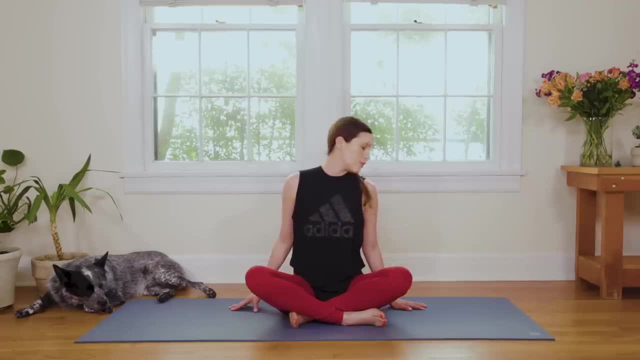 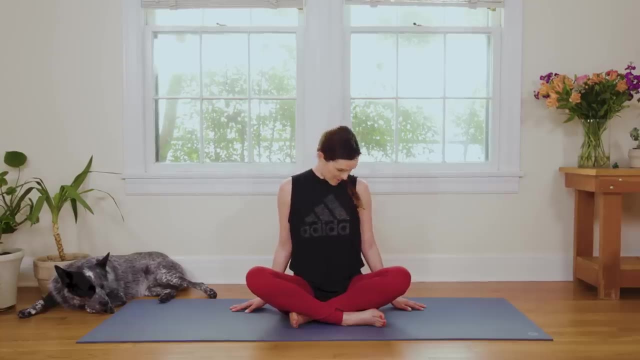 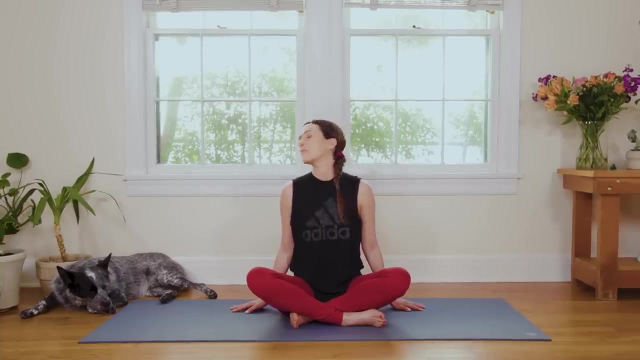 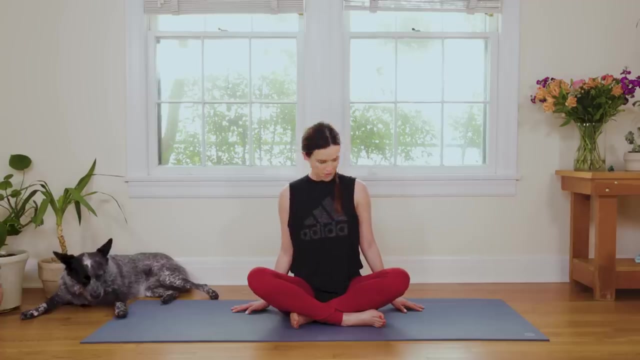 And then it gets a little bigger dinner plate, Frisbee And then like a big symbol. Okay, then reverse it. We're gonna start large and grow smaller. Daily neck hygiene- So important? Benji agrees. Alright, when you come back to center. 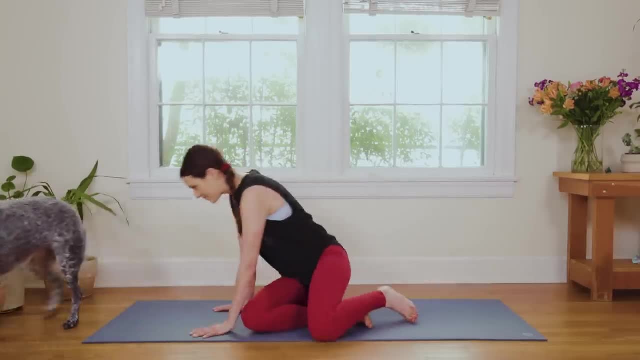 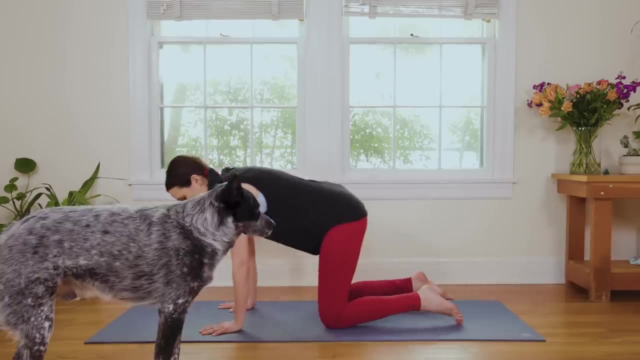 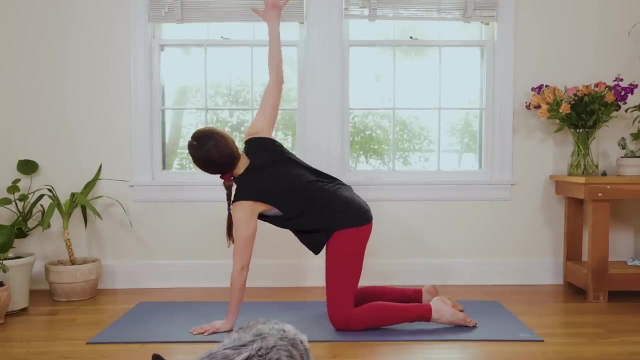 we're gonna take it forward and onto all fours. Hi, buddy, When you get there, take a deep breath in, A long breath, out On your next inhale you're gonna reach the right fingertips all the way up. Feel a nice big opening through the front body, front chest. 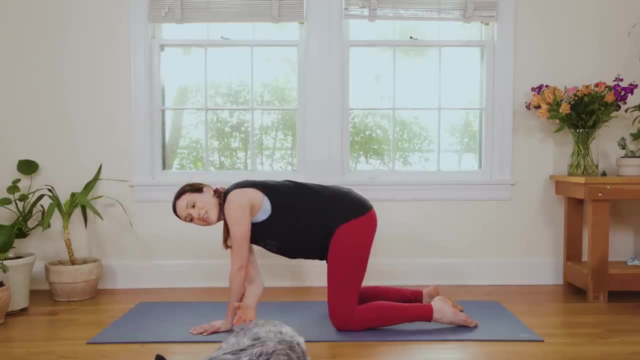 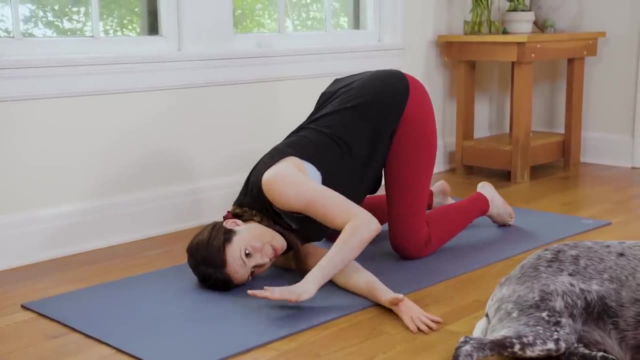 And then exhale, thread the needle. You're gonna take your right fingertips under the bridge of your left arm and we're gonna rest on the right ear. So yogi's choice here: you can press the left palm into the earth, left elbow. 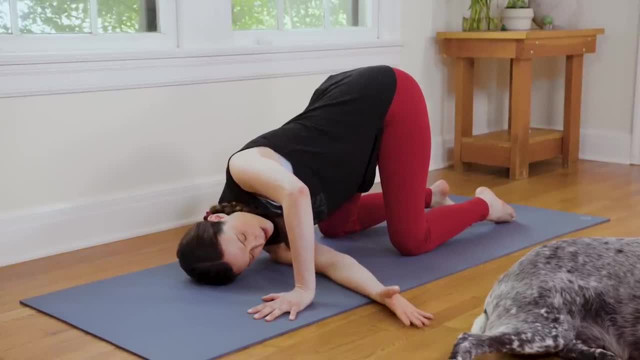 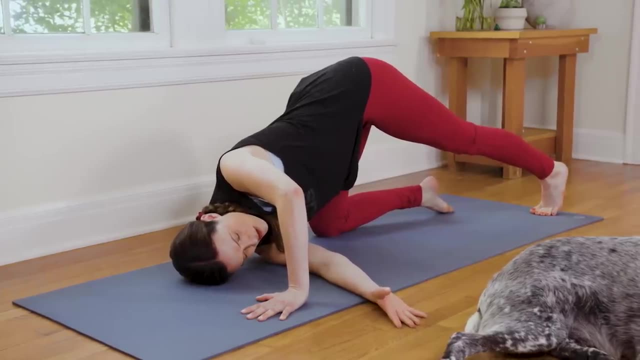 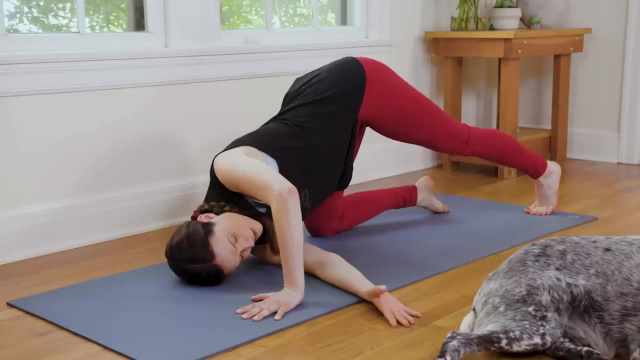 Give yourself a little connection here to find a deeper stretch in the upper back body. Another option is to curl the left toes under. Send the left toes back. Find a version that works for you today. Take a deep breath in, A long breath out. 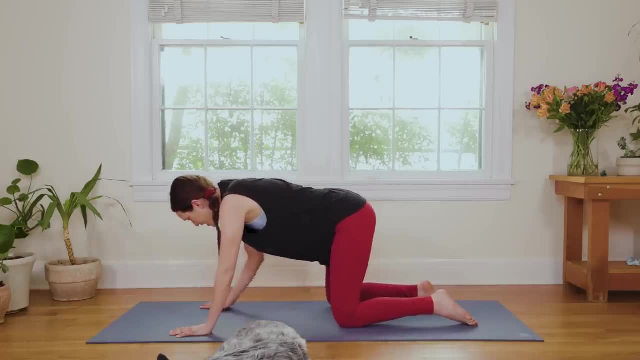 And then slowly unravel, Bring it back to center And we'll take it to the other side. One last twist. So really find your breath here, Inhale, open up through the front body, front chest, Left fingertips to the sky. 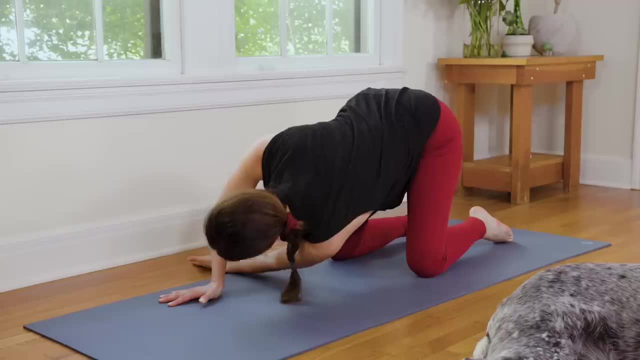 And then, when you're ready, exhale thread the needle Left hand to the left. Exhale thread the needle Left hand to the left. Exhale thread the needle Left hand to the left. Exhale thread the needle. 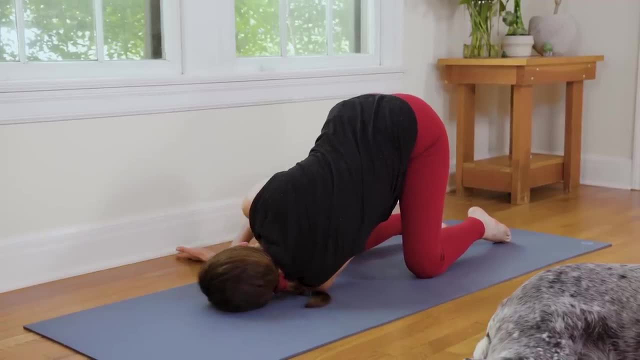 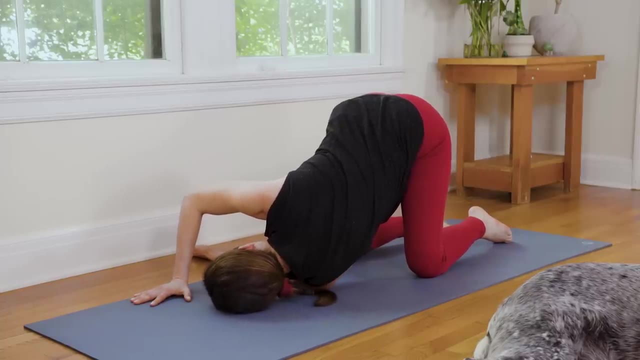 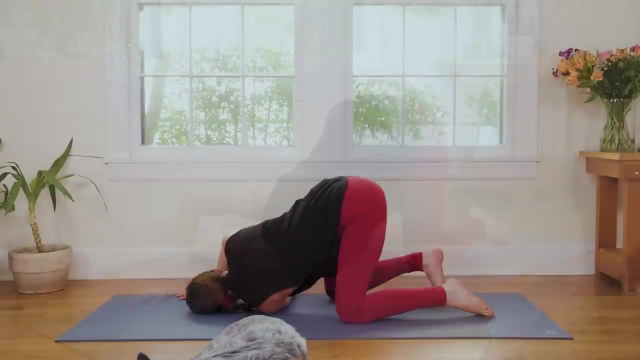 Left fingertips. go in and underneath the bridge of your right arm And same thing: Find what feels good with your right hand, Find that connection, Feeling, that opening through the back of the left shoulder, Upper back body And option, if it feels right in your body. 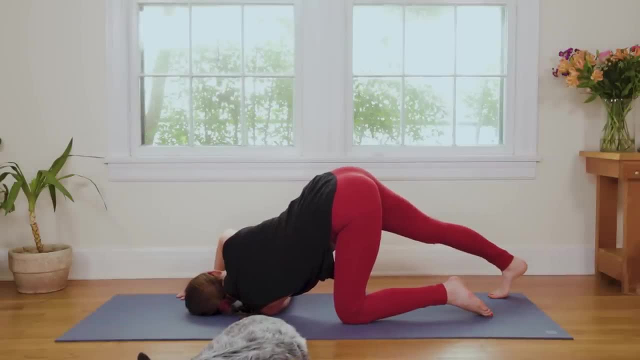 to curl the right toes under, Extend the right leg, Keep those right toes on the earth, Breathe deep, Take one more inhale, Inhale in And exhale out And then slowly unravel. Come back to center.